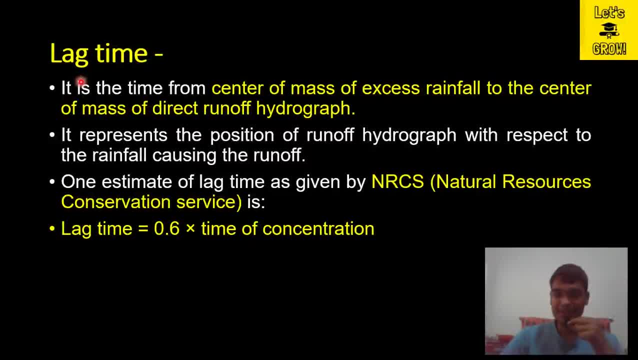 Hello everyone, welcome back to our YouTube channel. Let's grow. I hope you are very well and doing great in your life. So today's topic of discussion is leg time, That, what is the meaning of leg time and how it is calculated for a given hydrograph. So, without wasting, 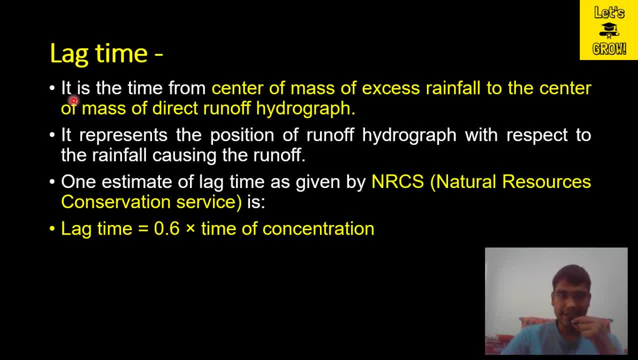 any time let us start our discussion. It is the time from center of mass of axis rainfall to the center of mass of direct run of hydrograph. So leg time is a time period between the center of mass of axis rainfall and the center of mass of direct run of hydrograph. So in the 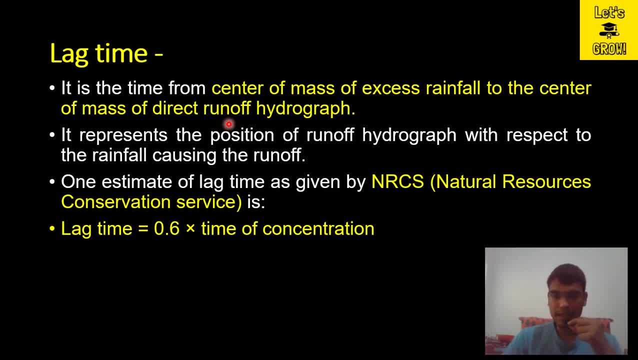 later slide we will use a figure for the better understanding of this statement. For the physical meaning, you can understand that late time is a time period whenever the peak precipitation or maximum precipitation is happening to the maximum discharge, or we can say peak discharge is observed at the outlet of. 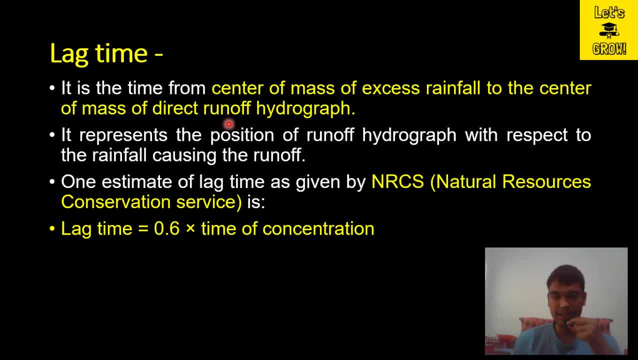 catchment. So what? our general belief is that whenever precipitation is maximum, at the same time we will get the maximum discharge. But this is not the case, because water takes some time to travel in the catchment, So there is some lag in the time whenever you get the maximum precipitation and when you get the 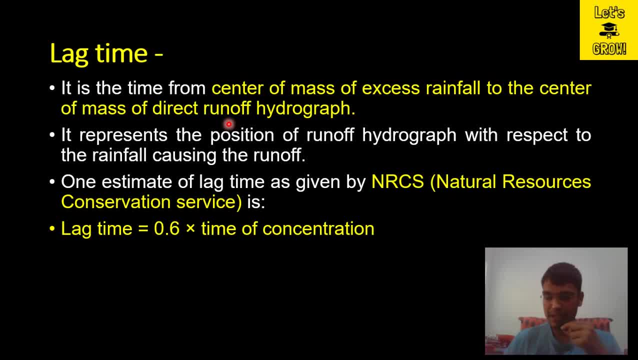 maximum discharge. So how much time it will take. between the maximum precipitation is happening to the maximum discharge, we are getting to the outlet. This is called the lag time, because the time is not the case, So the time is not the case. So the time is not the case. 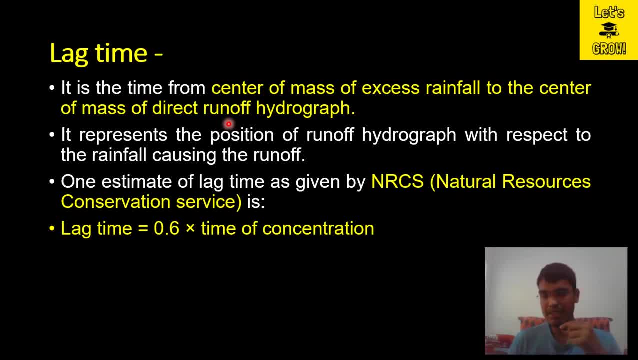 So the time is lagging between the maximum precipitation is happening to the maximum discharge we are observing at the outlet. It represents the position of runoff hydrograph with respect to the rainfall causing the runoff. So basically, it will show the position of runoff hydrograph with respect to the rainfall. 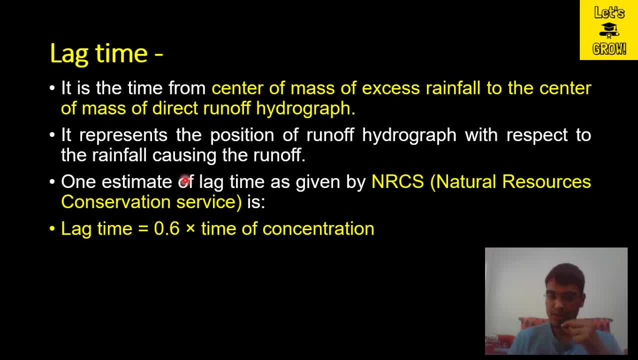 causing the runoff. So the position of maximum peak of rainfall to the maximum peak of runoff discharge will be based on the lag time. one estimate of leg leg time, as given by NRCS, which is natural resources conservation service, is that lag time is equal to 0.6 times of time of concentration. time of concentration we. 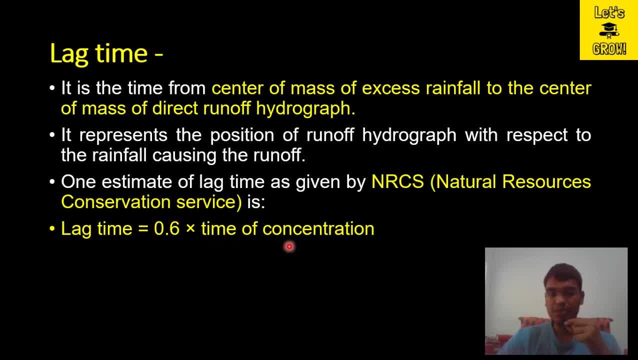 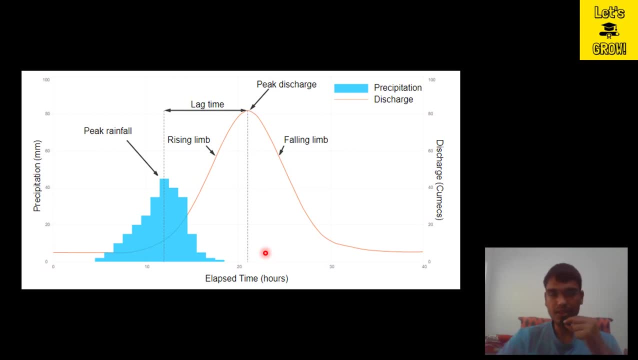 have discussed in our last video. so if you did not watch that video, I will request you to watch that video video so simply you can calculate. the lag time is equal to the 0.6 times of time of concentration. so here we are having this figure, so let's try to understand that how and what is the lag time? 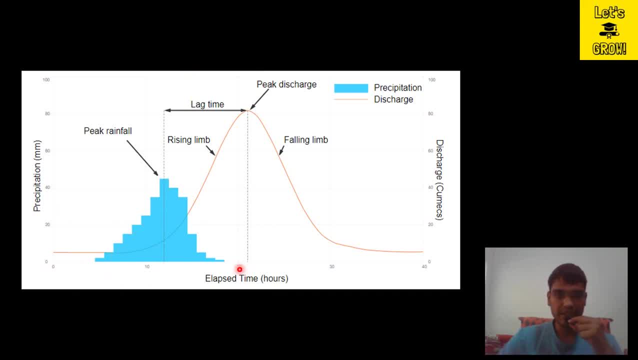 so here we are having the precipitation, with the time that how precipitation is is increasing with respect to the time, and there is a time when we will get the peak rainfall. so here you can see, this is the peak rainfall and due to the this rainfall event at the outlet of the catchment, 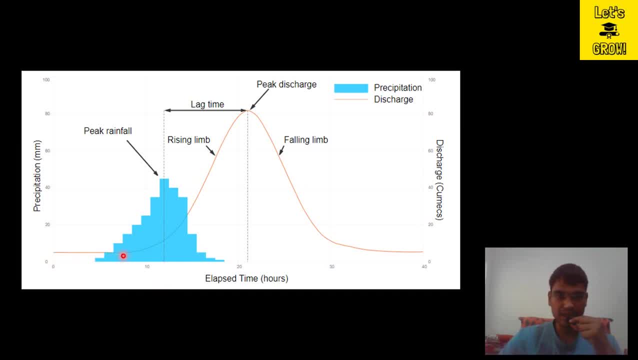 there will be discharge and this discharge is constant here and as the precipitation is occurring, it will increase, increased with time and it will attain some peak discharge and later on it will decrease. so this increasing of discharge is represented by this rising limb and this decrease in discharge is represented by the falling limb. so here we are getting the peak discharge. 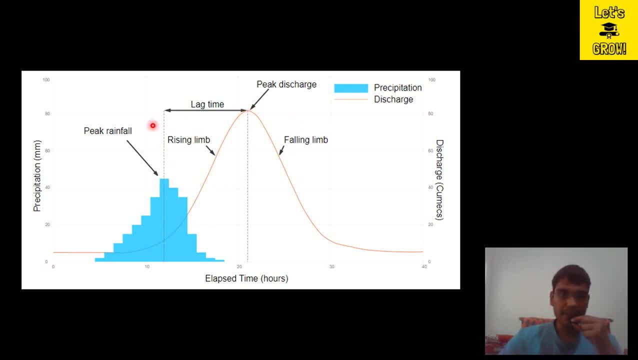 so this is the time period between the- when we are getting the peak rainfall- peak rainfall is here- and when- when we are getting the peak discharge, peak discharge is here. so if you measure the time period between the peak rainfall and peak discharge, it will give the lag time for that watershed and given precipitation event. 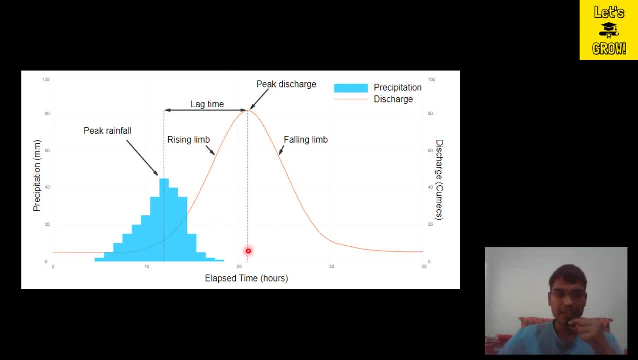 so i hope you understand this. and one more thing i would like to explain that why it is called as lag time? because our general belief is says that whenever we are getting the peak rainfall, the same time we should get the peak discharge. but this is not the case, because the 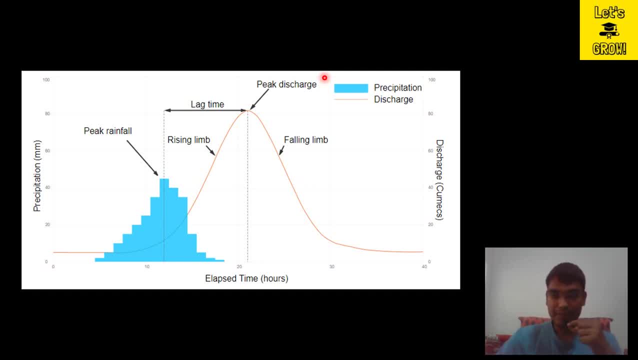 some time to travel in the catchment so this time is lagged by the catchment characteristics. So here, whenever this peak rainfall is happening, it will take some time to reach at the outlet so that it contribute to the peak discharge. So I hope you understand the concept of lag time. 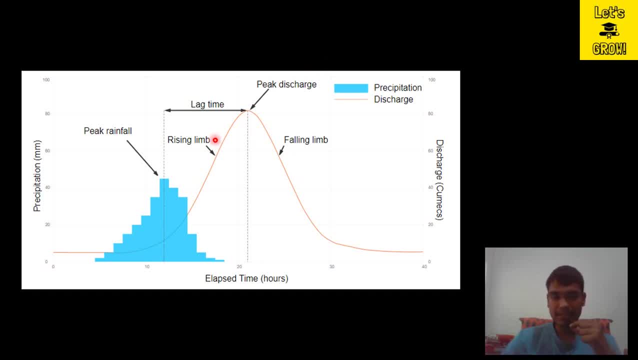 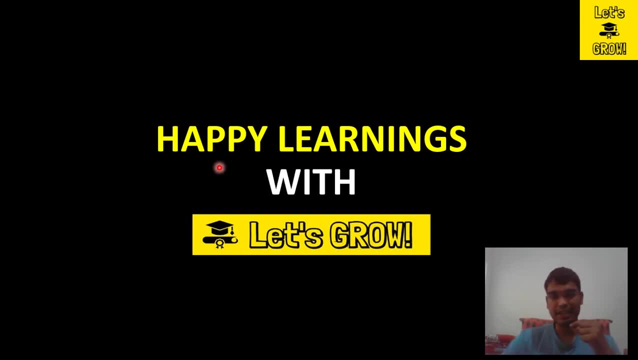 If you find this video informative, you can hit that like button. subscribe our channel. let's grow for more informative video. Thank you so much to watch this lesson till the end. ok, take care. bye, bye. 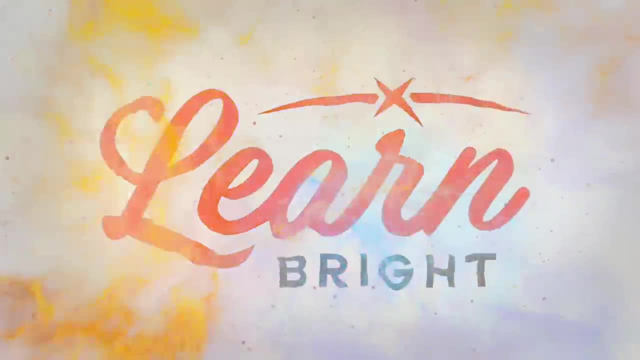 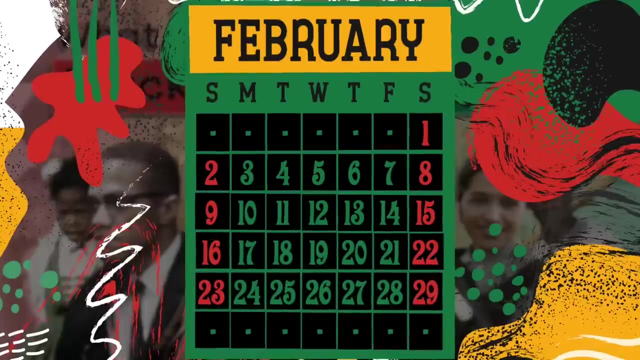 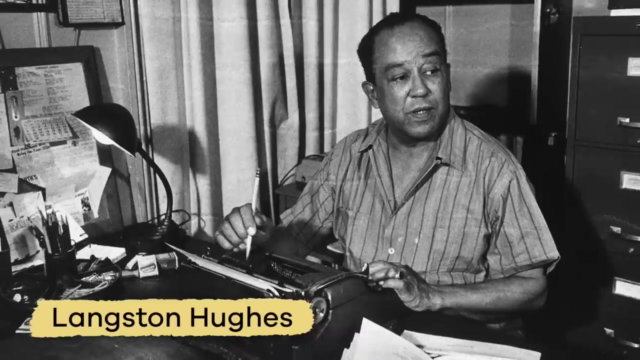 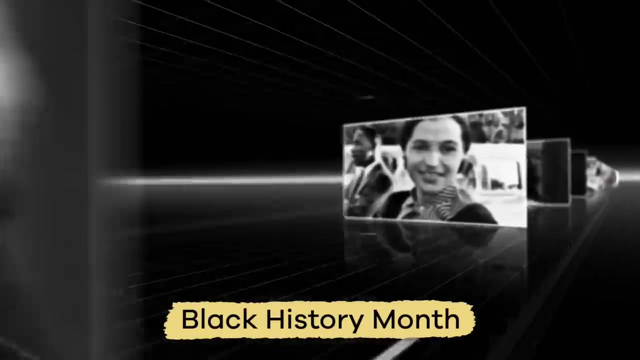 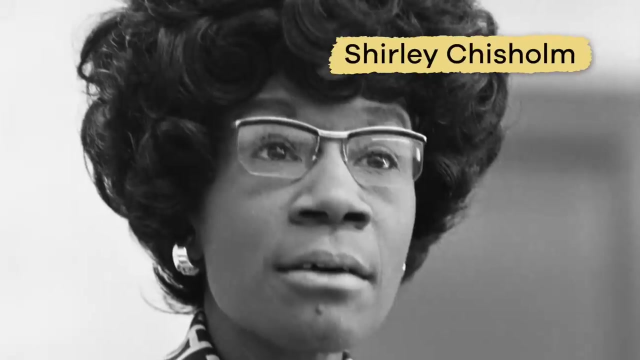 What is Black History Month? Did you know that every February, Americans celebrate the achievements of African Americans throughout history? This special month of reflection is called Black History Month, And today we are going to learn more about what it is and why we celebrate it every year. You have probably heard the names: Martin Luther King Jr. 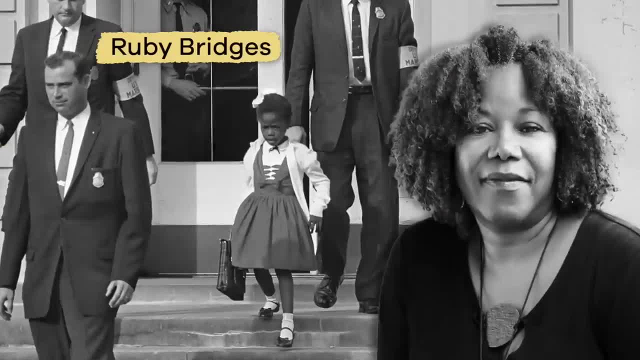 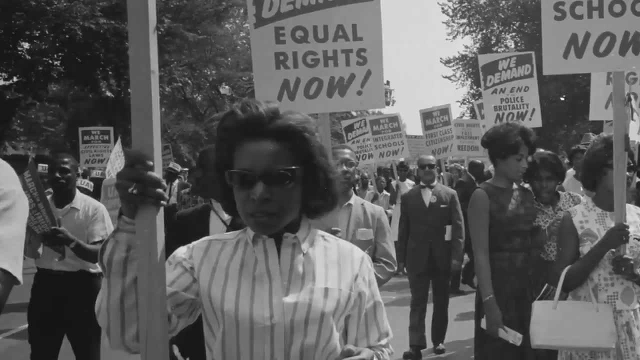 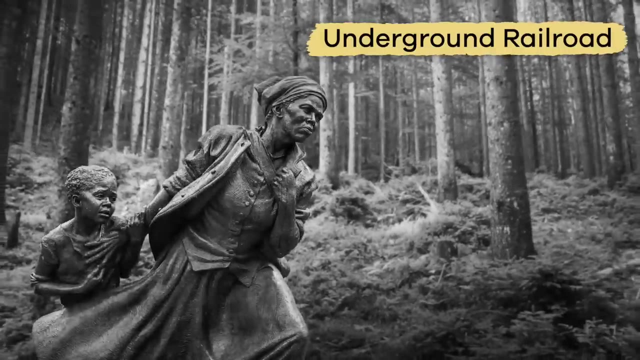 Rosa Parks, Malcolm X and Ruby Bridges before and learned about their roles in the civil rights movement. You have also probably learned about Harriet Tubman's courage during the Civil War and her role in the Underground Railroad, But the history of African Americans in the 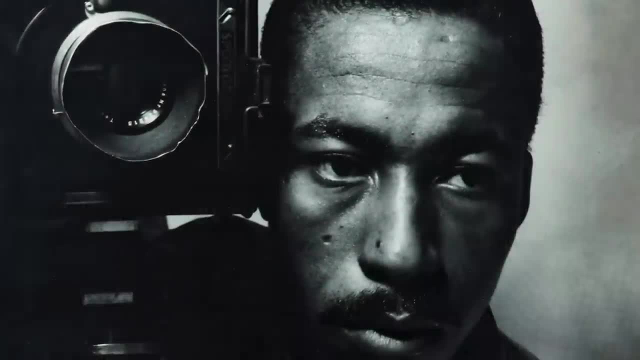 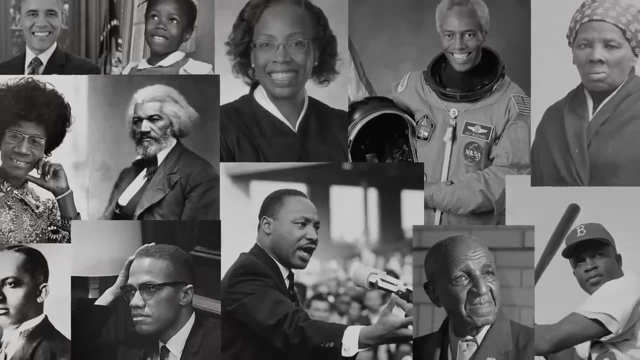 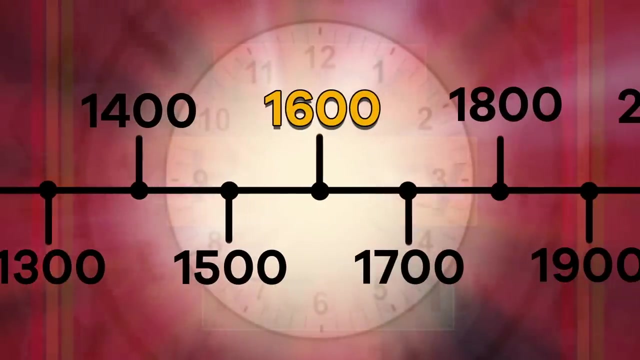 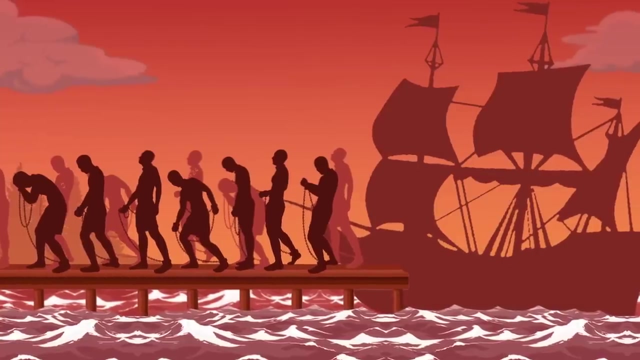 United States has not always been so available, which is why Black History Month is so important. To understand more about the origins of Black History Month, we have to go back in time, way back to the 1600s. In 1619,, European colonizers brought 20 enslaved Africans to. 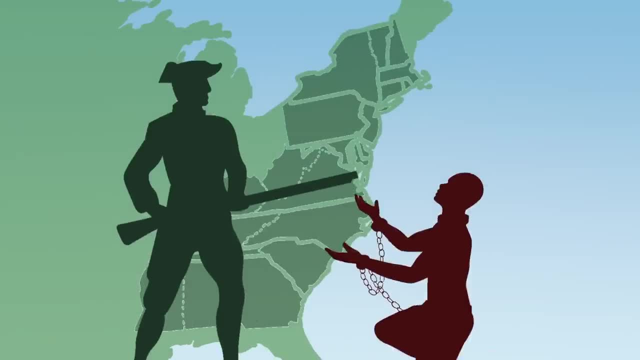 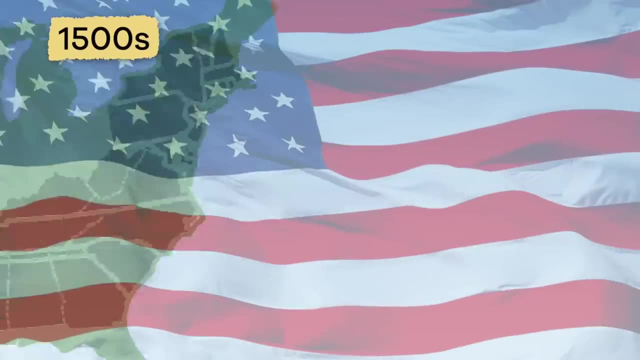 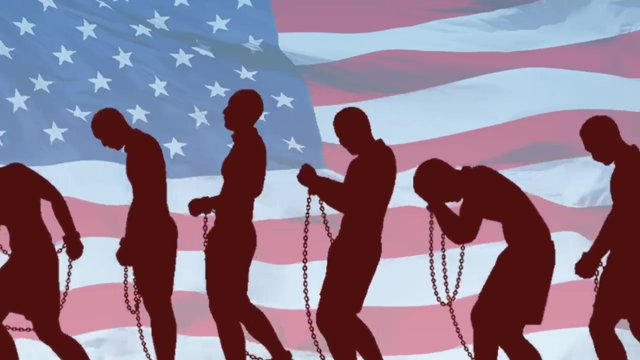 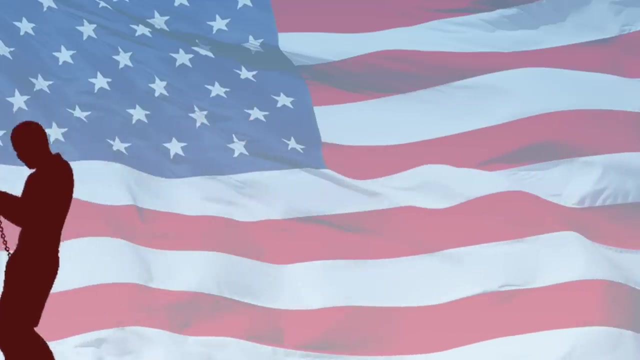 the mainland American colonies And many historians believe that the practice, meaning the process of life, happened here in the United States. 쁨 that you are an American now is a Demonstration of Brexit values and roots as well as imperial value. This was not a faceless description of the Zhelga New Testament, But it was a thinking.